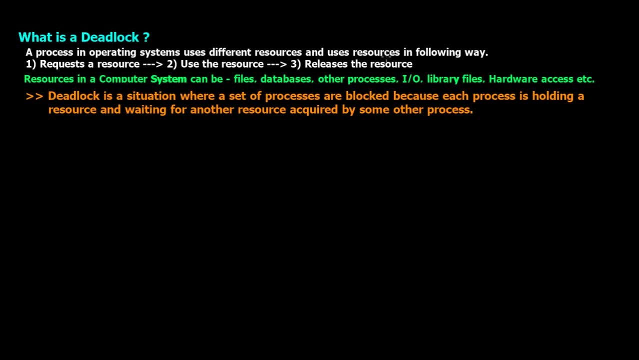 So process in operating system uses different resources and uses resources in the following way. So whenever a process is running in the background or in the foreground, or whenever you're opening an application, closing an application, using an application, there are a number of processes that are happening in the background and these processes access. 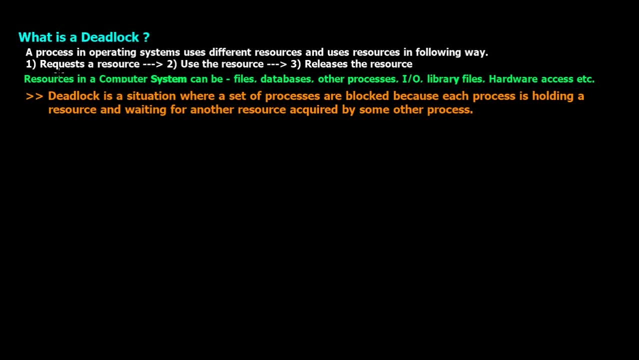 certain resources on the system right. So the first step is the process request for that resource, Then the process uses that resource And lastly, it releases that resource. So this is what happens, step by step, whenever a process is going to access a resource right. 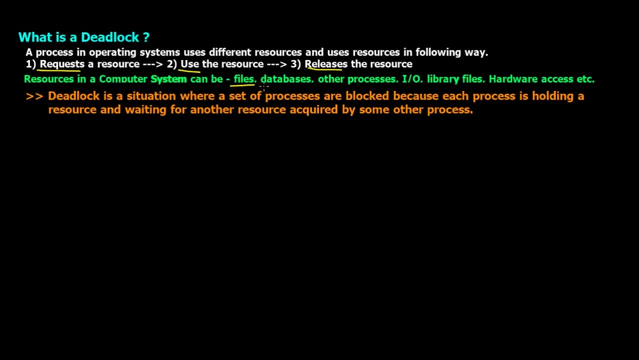 And resources in a computer system can be files, can be databases, can be other processes can be input output operations can access certain library files, or a process wants a hardware access. For example, if you are connected to a printer, maybe a process wants. 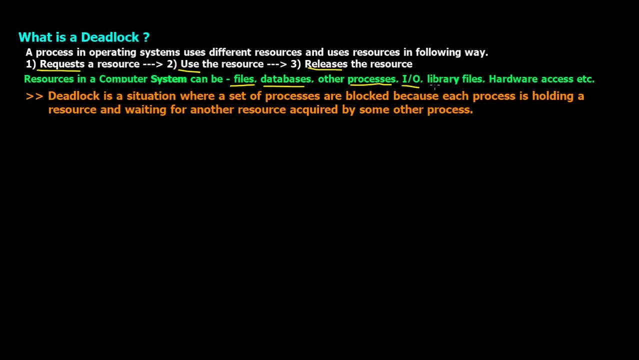 to print certain pages, and so on and so forth. So there can be a number of different types of resources in a computer system which a process might want. Now, deadlock is a situation where a set of processes are blocked because each process is holding a resource and waiting. 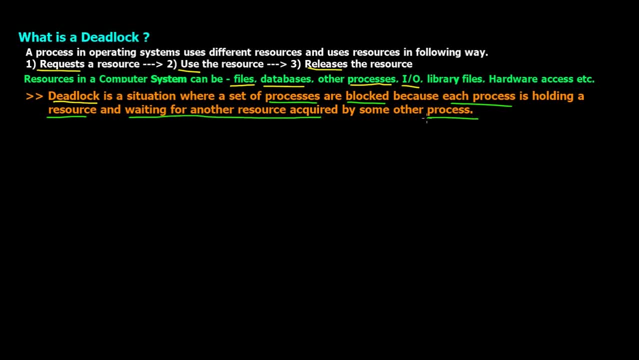 for another resource acquired by some other process. Now, if you read it for the first time, it might not be that clear. So let's see a real world scenario for deadlock which happens in our day-to-day lives. Okay, So this is a basic scenario of a deadlock. So 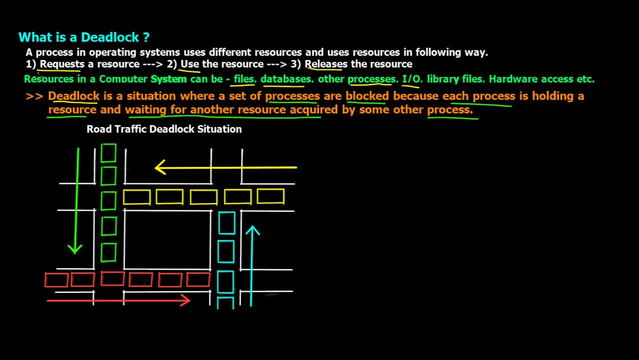 scenario of a road traffic deadlock situation. so, as you can see on the diagram, these rectangular boxes in different colors are basically cars. just assume that they are cars. and these white lines are basically roads. now you can see that these green set of cars are traveling in this. 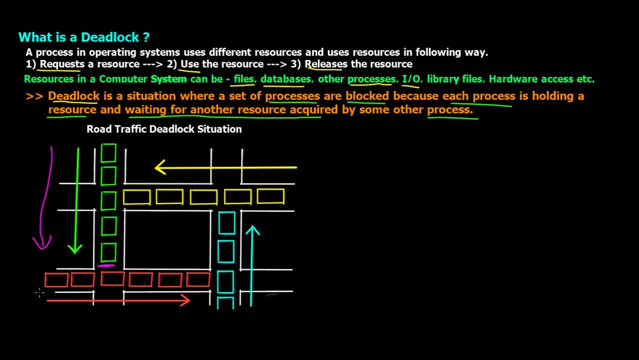 direction. they are blocked over here because there are different set of red color cars which are traveling in this direction, starting from left to right. again, these red color cars are blocked over here by blue cars which are traveling from bottom to top direction. the blue color cars are blocked. 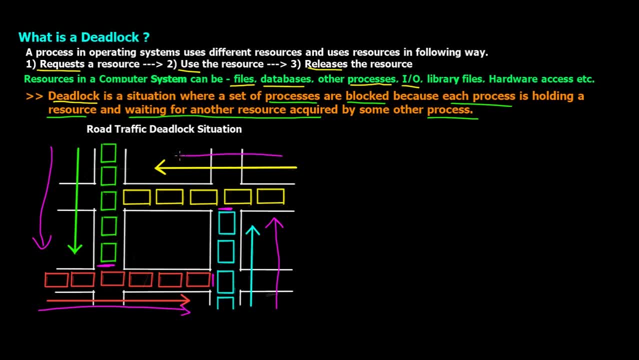 over here because of these yellow cars which are traveling from right to left. now this is a situation of a deadlock in real world scenario and if you are specifically from mumbai or a city in india which is heavily populated, this is our regular situation. it's not nothing new to us. but 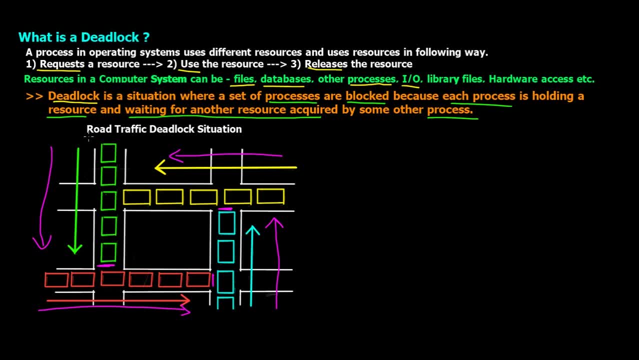 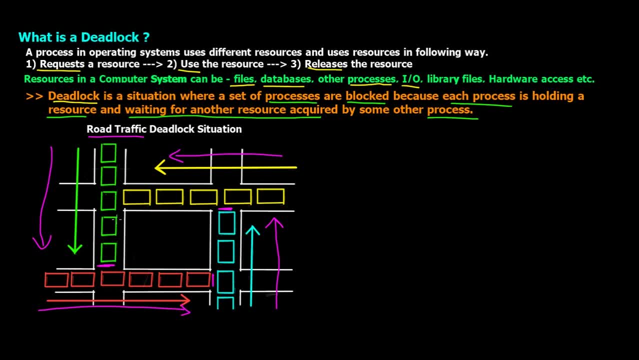 because all of them are blocked by some other cars. the green ones cannot move ahead because they are blocked by red. red ones cannot move ahead because they are blocked by blue. the blue ones cannot go ahead because of yellow and yellow can't go out because of green. so basically, this becomes: 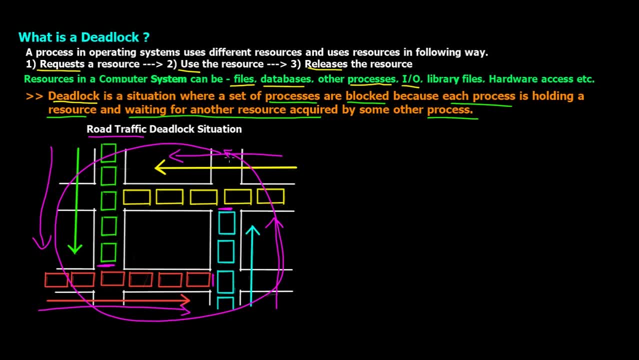 a complete circular cycle where every car is waiting for other car to move ahead, but they cannot move out because they are indirectly blocking each other itself. so now, taking this real world scenario into mind, let's see what happens in an operating system scenario. okay, so a diagram for an operating system deadlock situation. it's a very simple diagram, so in the 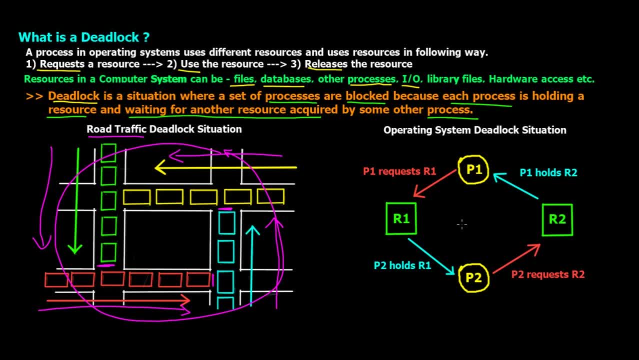 yellow circles. we have process p1 and process p2, so this p1 is process 1, p2 is process 2. in the green square boxes we have resource r1 and resource r2, so this might be something like files, this might be something like a database, and so on. okay, now here's a situation: p1 holds r2, which means that 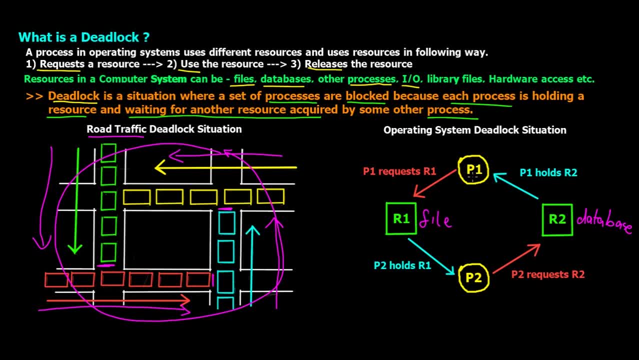 this database r2 is already assigned to p1. it's already assigned to p2, so it's already assigned to p1. okay, so p1 has complete access of this database r2. but p1 now wants r1, which is a file. okay, so let's say, p1 is a process which copies certain values from the database and is going to print. 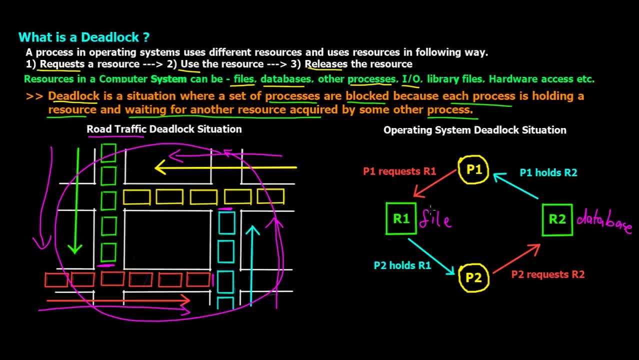 it in the file. so that's why p1 wants access of the file. but p1 is not able to access r1 because r1- that is, this file- is allocated to p2, so p2 holds r2. okay, now p2 wants control of the database. 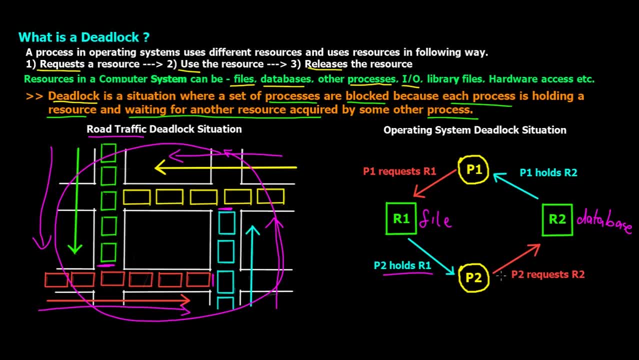 that is resource 2. so p2 requests for r2, but p2 cannot access r2 because r2 is assigned to p1. so you can see that there is another circular pattern going on over here. and p1 cannot access r1 and p2 cannot access r2, right, because each of them are assigned to either of the two processes. 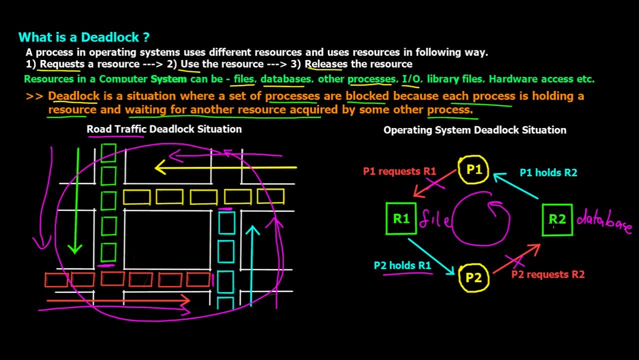 respectively. that is, p1 has control of r2, so p2 cannot access it, and p2 has access of r1, so p1 cannot access it. so both of them are assigned to r1 and p2 cannot access r1, so p1 cannot access it. 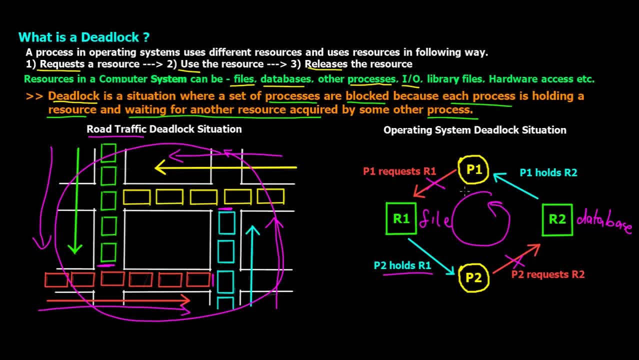 both of them are in a deadlock situation wherein they are waiting for each other to release those resources so that they can access it. so this was a deadlock situation, a very basic deadlock situation in our operating system scenario. so i hope you have a overview about what is a deadlock. 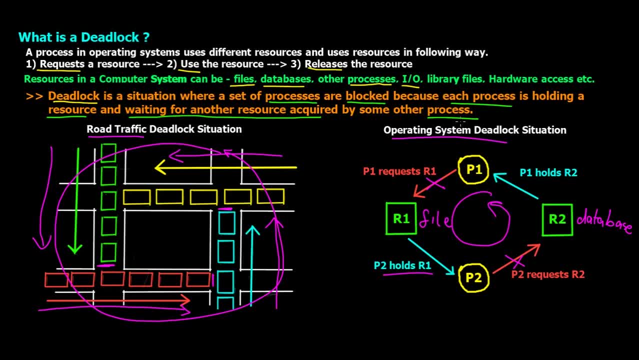 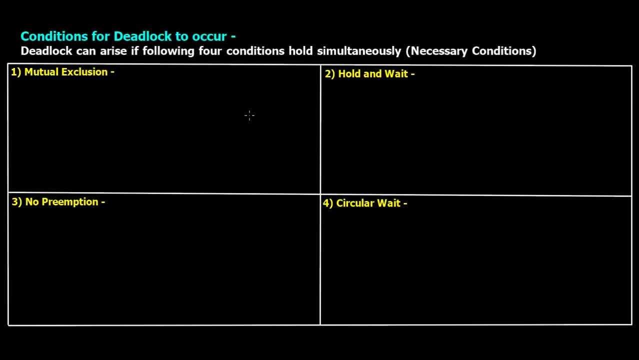 and how it happens in operating systems. but now let's understand in detail what are the particular conditions that needs to be true for a deadlock to happen in an operating system scenario. okay, so, as you can see on the screen, we have four conditions which needs to be true simultaneously. 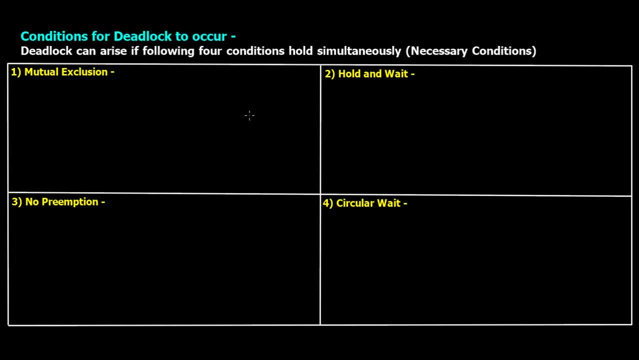 for a deadlock to happen in your computer system, in your operating system. so what are those four conditions? so the first one is mutual exclusion. second one is hold and wait. third one is no preemption and fourth one is circular wait. now, these are very important conditions which you 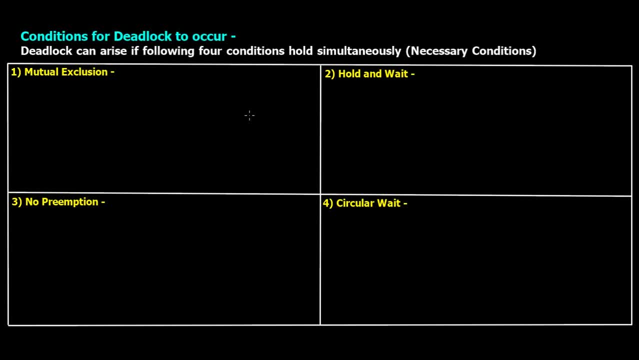 definitely need to understand, and if you are making some notes, you can probably note down each of these in your book. and now we'll discuss each condition in detail individually. so let's start off with mutual exclusion. so, in mutual exclusion, one or more of the conditions that 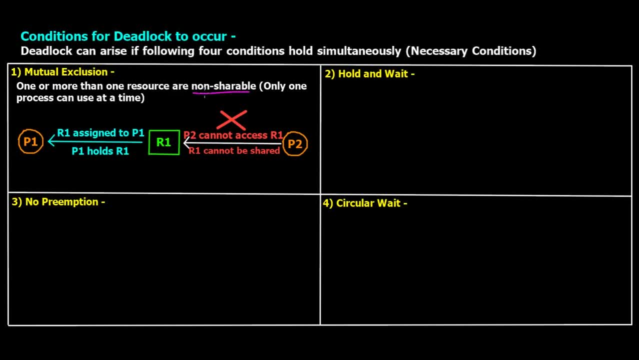 more than one resource are non-shareable. that is, only one process can use it at a time. so here's a scenario: we have process p1 and we have process p2. we have one resource, r1, over here. now r1 is assigned to p1, which means that p1 has access of r1. now, since the concept of mutual exclusion, 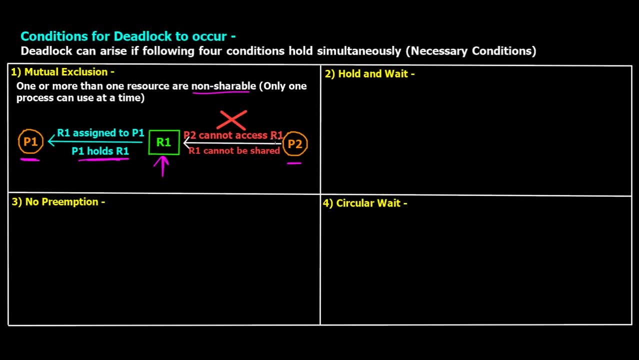 exists. this means that p2 cannot access r1 and r1 cannot be shared. so until and unless p1 releases the access of r1, p2 cannot access it, right? so p2 is going to be waiting for r1, so this can lead to a deadlock situation, right? so in the previous diagram of 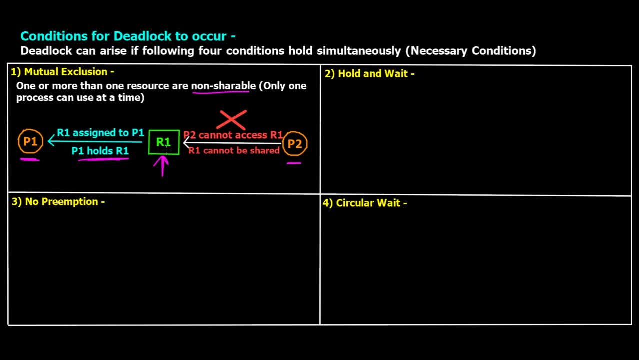 that deadlock situation in operating system. this was exactly happening, right? that is, each process was waiting for a particular resource which the other process was already holding, right? so this is that mutual exclusion condition. now let's see what is hold and wait. so in hold and wait, a process is holding at least one resource, so it can hold more than one, but it is holding at 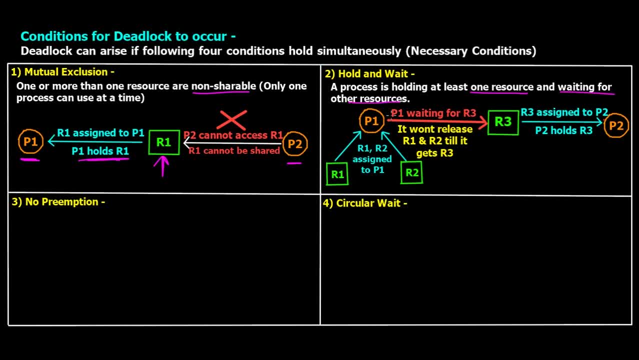 least one resource and is waiting for other resources too. so let's see what is hold and wait here diagram and understand this in more detail. so again, we have p1, which is process 1. we have p2, which is process 2. now p1 already has two resources, so it is holding r1 and r2. okay, so r1 and r2. 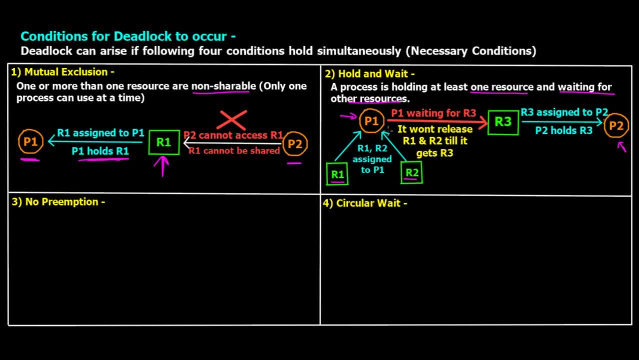 assigned to p1. right now p1 wants a third resource, r3. so p1 is waiting for r3 and it won't release r1 and r2 till it gets r3. but r3, that is, this resource r3 over here is assigned to p2, so p2 holds r3. 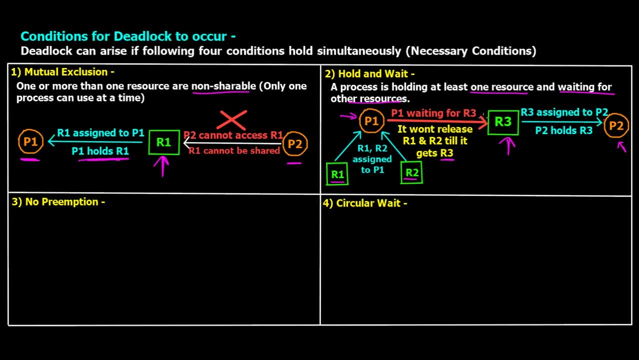 so, since p2 is holding r3, p1 cannot access it and it is waiting for r3 because of this mutual exclusion condition, and p1 is waiting for r3. so because p1 is waiting for r3, p1 will not release r1 and r2, even if the work of accessing this resources is done. so this is what this yellow 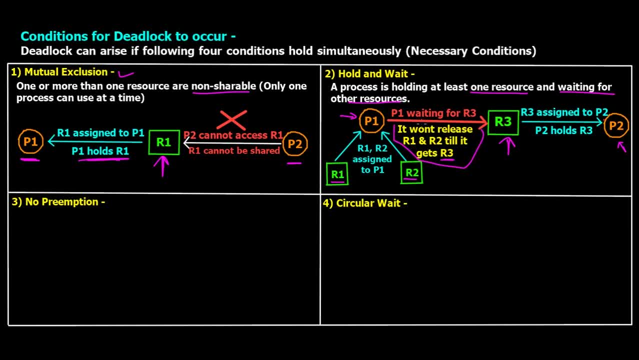 statement says it won't release r1 and r2 till it gets access of r3. so this is that hold and wait condition. so it's holding r1 and r2. that is, two resources, but it is waiting for r3, which means that even if the work of r1 and r2 is done by p1 and, let's say, there is another, 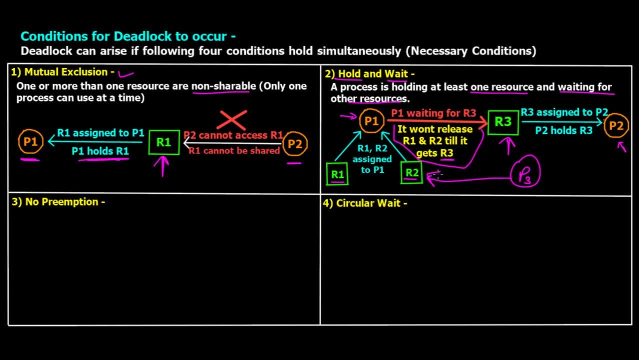 process. p3 wants access of r1 and r2. p3 will not get that access of r1 and r2 until p1 gets access of r3, which is held by p2. so then p1 goes into a deadlock situation of waiting for r3 and 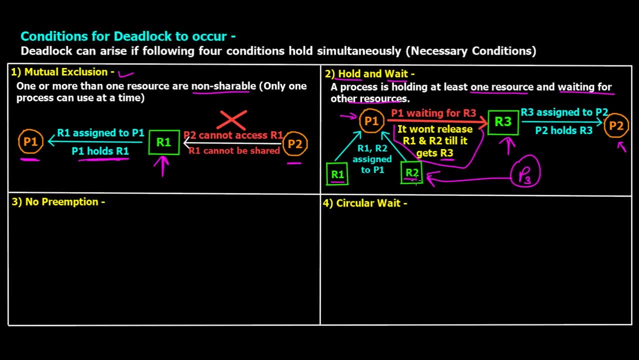 p3 also goes in a deadlock situation for waiting for r2 right, and this is just because of one resource being held by p2. so i hope you understood what is hold and wait. so let's see the third one. that is no preemption now. as the name suggests, preemption means preempting a. 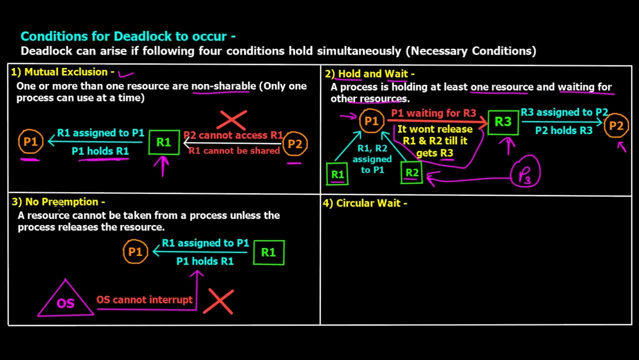 particular process, which means stopping a process in between. okay, that is the literal meaning of preemption in operating systems. so whenever you say i preempted my activity, which means that you exited your activity or stopped your activity in between, so no preemption means you cannot stop an. 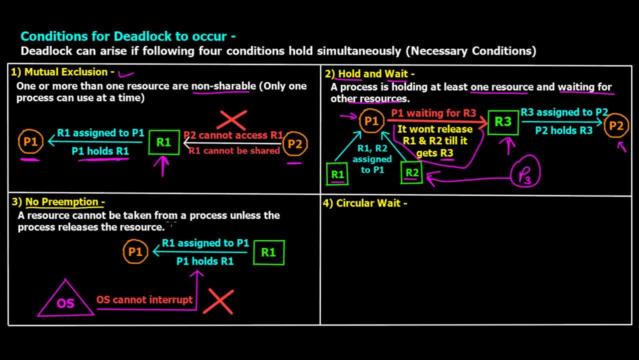 activity in between. so this states that a resource cannot be taken from a process unless the process is taken from a resource. okay, this makes sense, right? it's pretty simple to understand in text, but let's see diagrammatically what is happening. so here is a process, p1. now p1 is holding a. 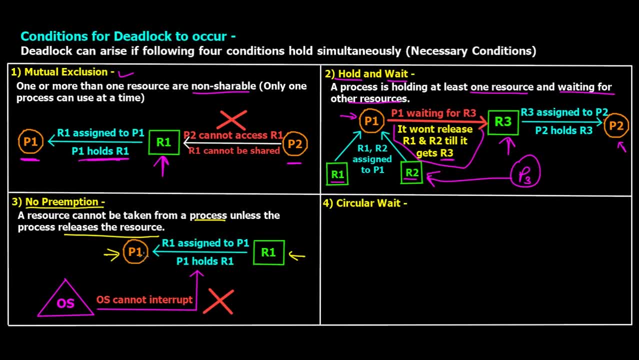 resource r1 over here in green. okay, so r1 is assigned to p1, or in other words, you can say: p1 holds r1. now, if there is no preemption, nothing else can stop or make p1 release this resource until unless p1 finishes it or decides to release it. so here's a scenario wherein there is a third. 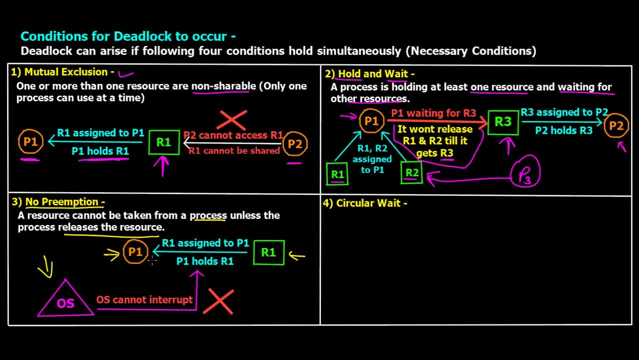 operating system, and operating system wants to stop p1 from holding this r1, but os cannot interrupt now because there is no preemption condition. so this is a third party which wants to stop p1 from accessing r1, but it cannot do so because we have no preemption. okay, so this is that meaning of no. 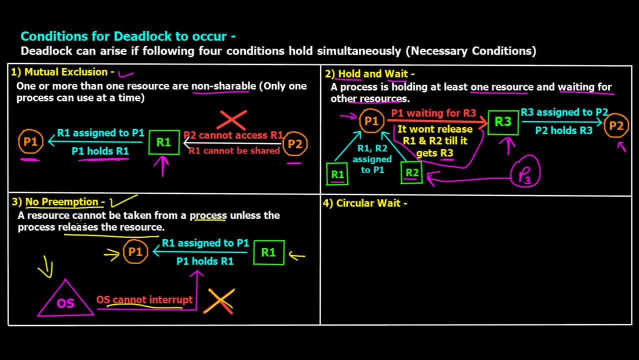 preemption, which means a resource cannot be taken from a process unless the process releases the resource. so it is on this process to release this resource r1, when it feels that it has completed its activity. so this can lead to a deadlock situation. so what if the process p1 doesn't release r1 ever? so if 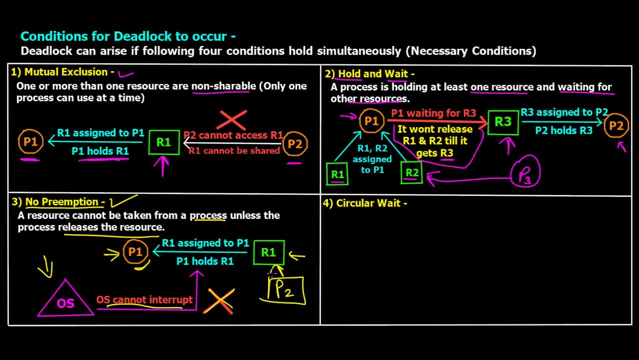 there is certain other process: p2. it will never get access of r1, even if it wants to right, because of mutual exclusion. so again, non-preemption or no preemption results into deadlock scenarios and let's see what is the last scenario, that is circular weight. so this is that diagram which we 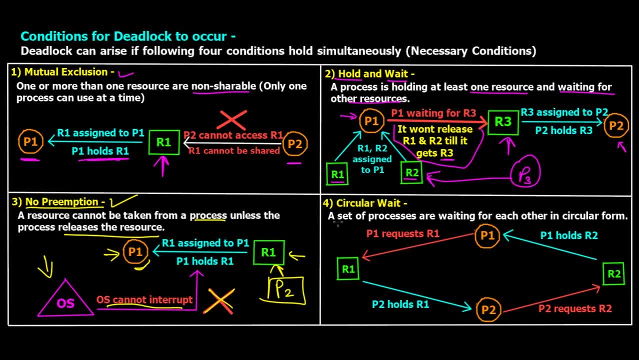 saw of deadlock situation in the previous slide. so in circular weight a set of processes are requested to Hong Kong. there's also a bit of trigger when there's a request- for in some cases people say nobody knows what's what for something- tab is available. so the b2 request we say we need to see that's when r1 will not be accepted. 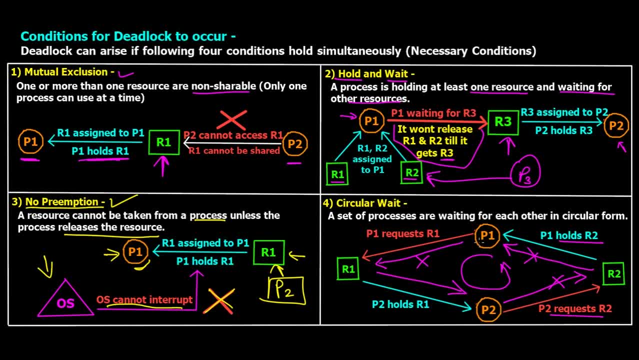 because they have access to other resources, that is, they have access to opposite resources which they are requesting for right. So this is that circular wait scenario. So these are the four very important conditions for a deadlock to happen in an operating system scenario, and I hope you. 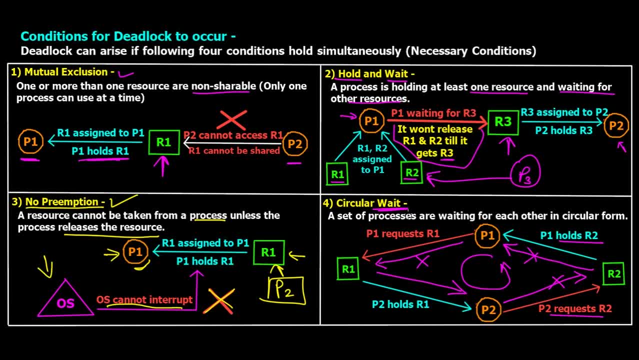 have a very good idea about all these four conditions. You can probably note these points down and you can also draw these diagrams for better understanding. So now let's move ahead and see some important strategies and important ways in which a deadlock can be prevented, or a 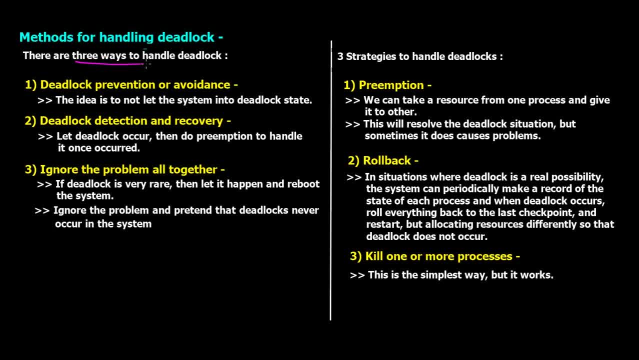 deadlock can be recovered from. So in general, there are three ways to handle deadlocks, and then there are three other strategies also which can be used to deal with deadlocks. So let's discuss first the three ways to handle deadlocks. Now the three ways are deadlock prevention or 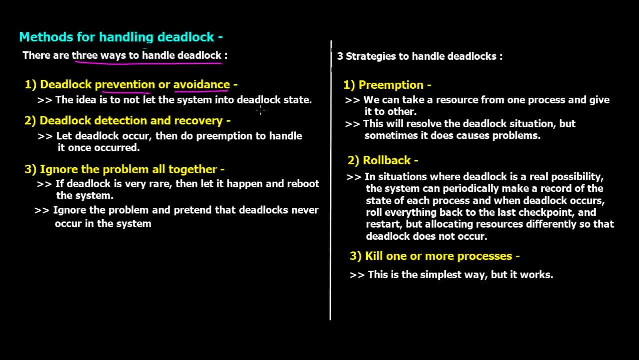 avoidance, which means that the idea is to not let the system into a deadlock state itself. So even before the deadlock happens, you predict that there is going to be a deadlock happening, depending upon those conditions that we discussed in the previous slide. So if those conditions are, 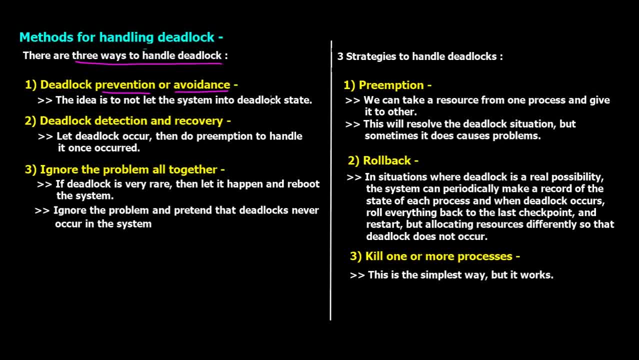 going to be true. you make certain calculations and you avoid the deadlock happening itself. Okay, so this is step number one, or this is method number one? Method number two is deadlock detection and recovery. So what if you are not able to prevent the deadlock? you are not able to. 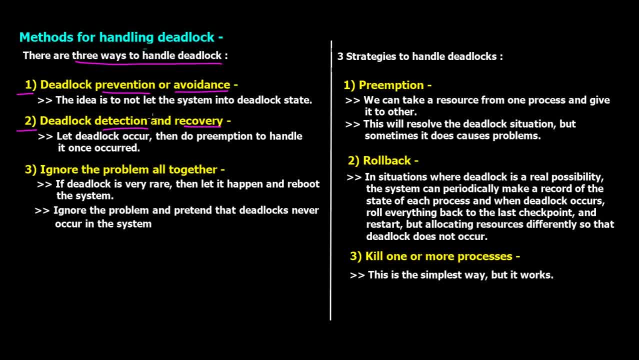 avoid the deadlock? and what if a deadlock has actually happened? So the next method would be to actually detect that there is a deadlock happening, right? So the system has to detect that there is a deadlock happening, and what if a deadlock has actually happened? So the next: 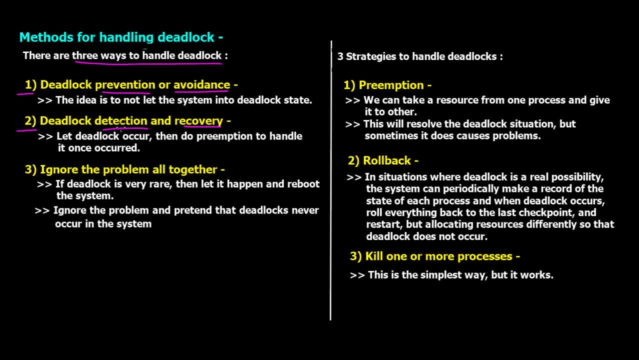 okay, this process is waiting for a resource for a long time. so let's see if there is a deadlock or not. so that is deadlock detection. and then, once detected, what are we going to do about it, to recover from the deadlock, to resolve that deadlock? so in this, we let the deadlock occur, but then we 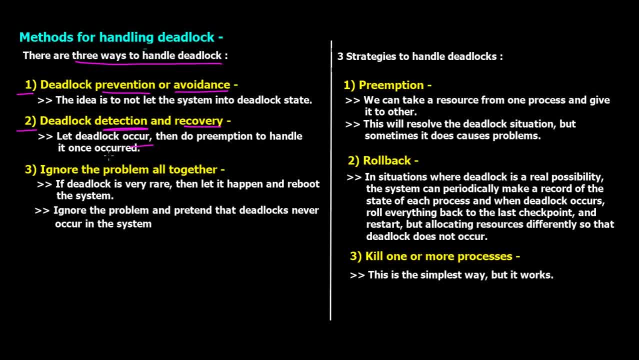 do certain techniques like preemption or rollback, to handle it once it is occurred. okay, so this is the different strategies and we'll come to that in a minute. and the last method is to ignore the problem altogether, and yeah, this is a pretty careless way to put it, but then if the deadlock 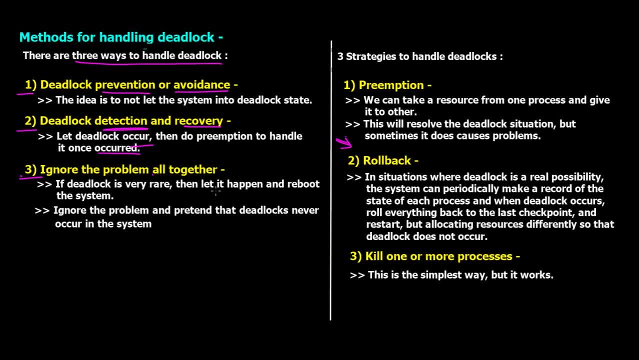 is very rare and the operations are not critical, then just let the deadlock happen and reboot the system. so this is not usually the scenario in real world cases. you need to have a system in place which prevents or avoids deadlocks, or at least detects and recovers deadlocks. okay, so in this, 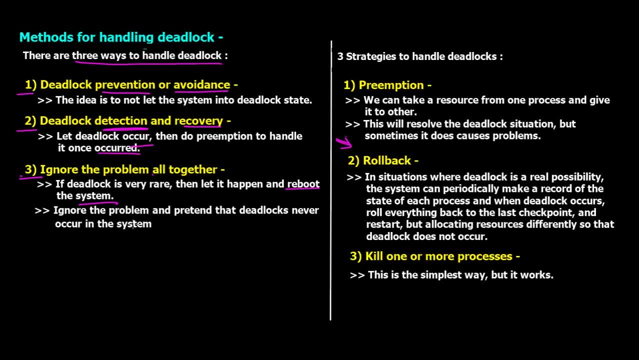 third step: we just ignore the problem and pretend that deadlocks never occurred in the system and just reboot the system. so this is very easy. but then in the real world scenarios, when the task and processes are critical, you do not do. step number three now. the strategies, as i mentioned, to handle deadlocks are preemption. so what if a deadlock?